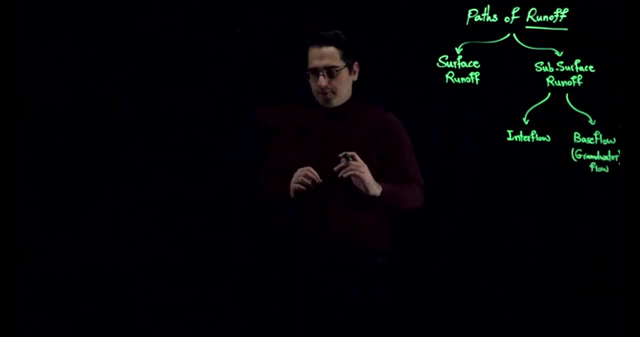 let's talk about hydrograph and what a hydrograph is. To help me to do this, I'm going to use a graph. I'm going to use a graph. I'm going to use a graph To help me to define a hydrograph. I am going to show you a sample watershed. 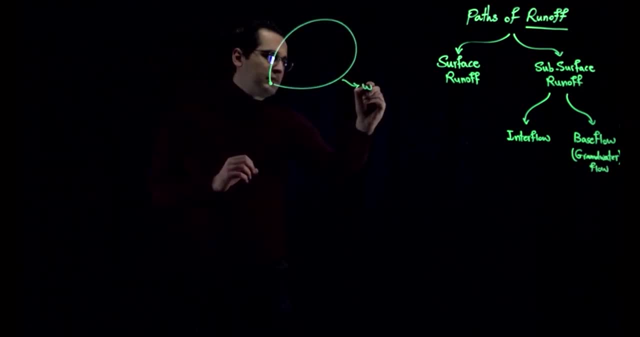 This is a sample watershed. These are the watershed boundaries And this point over here is the outlet of the watershed. Now let me show you the dendritic river network in this watershed. This is going to be the outlet of the watershed, So if you have any water in this watershed, the dendritic river network is going to collect. 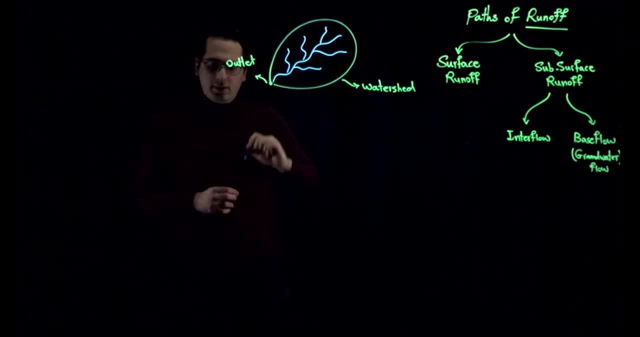 that water, and that water is going to be collected at the outlet of the watershed. We are going to have a gauging station right at the outlet of the watershed that measures the flow of water out of this watershed. I want to talk about this now. 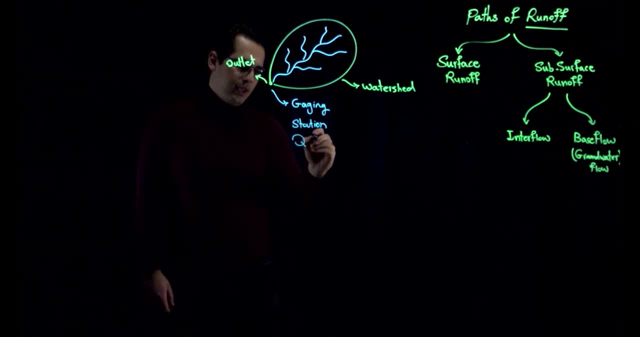 I talked about the flow of water. I'm going to show you by Q, And usually the units for this Q would be volume divided by time, So cubic meters per second or cubic feet per second Volume divided by time. Okay, So we have a gauging station right at the outlet that measures the flow out of this. 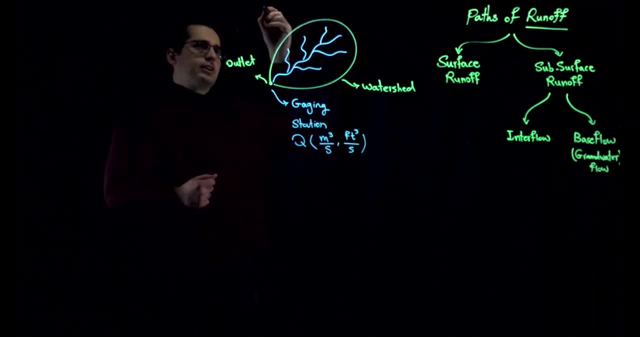 watershed. All right, Now let's say that we have a rainfall event and I'm going to show the rainfall event over this watershed. These are the clouds, All right. So this is the rain over this watershed. This rain is going to generate some flow. 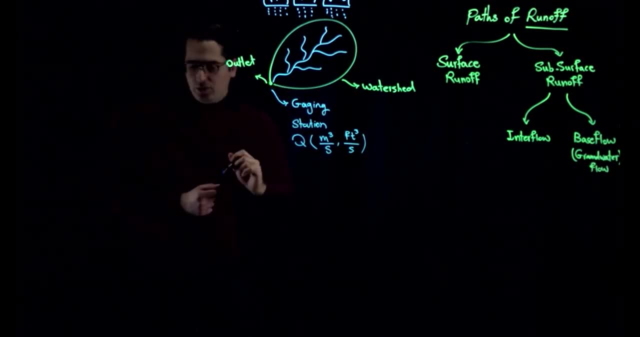 And at this point, we are going to measure that flow using the gauging station that we have. Okay, So what I'm going to do, I am going to show you the graph that we are going to have On the x-axis. we are going to have time. 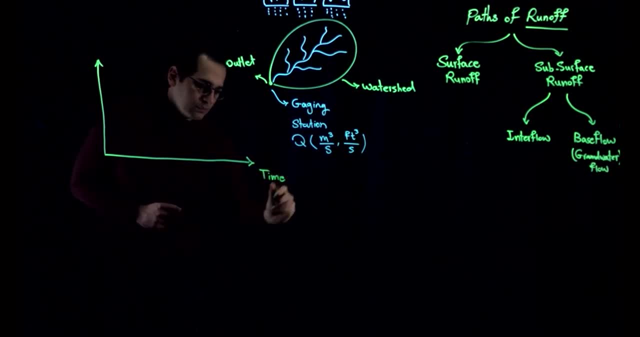 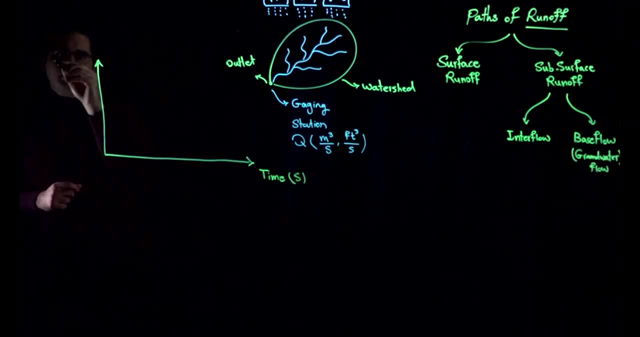 We are going to have time, So we are going to have time in minutes, hours, whatever, And on your y-axis you're going to have discharge or Q stream flow And this is going to be volume divided by time, Right. 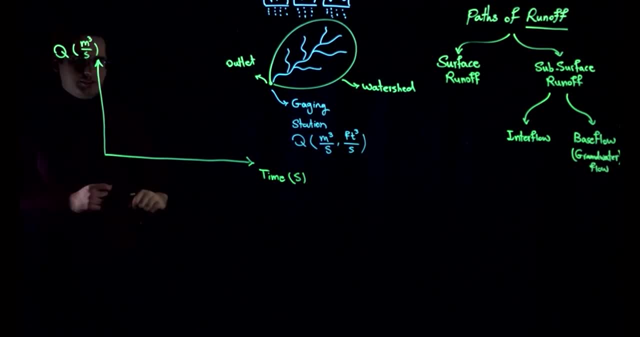 It's flow. So I'm going to say, let's say, cubic meters per second. as an example, Before the rainfall, let's say that the flow was something like this: This is before the start of the rainfall. As the rainfall starts, I'm going to show the rainfall by a block. 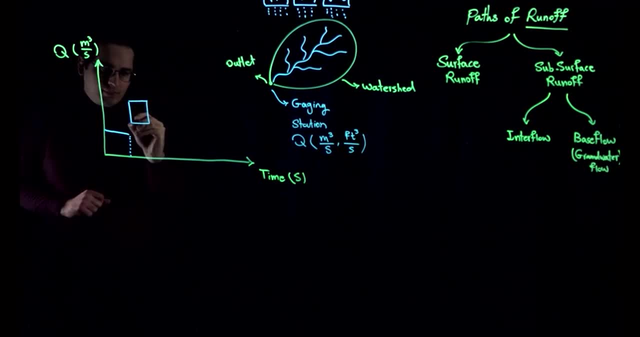 this is the block of rainfall. let's say that the rainfall is, the duration of rainfall is going to be T sub R and the height of this rainfall is going to be P in depth. so this is the rainfall over your watershed. as the rainfall starts, understandably, initially the parts of the 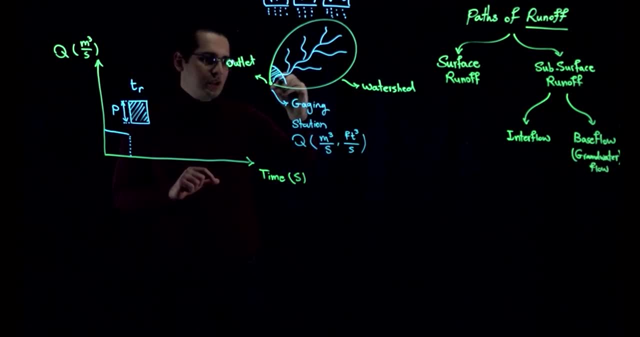 watershed that are closer to the outlet are going to contribute water, contribute flow to the outlet. so slowly this line is going to increase as different parts of the watershed that are closer to the output are contributing, then after that, other parts are contributing flow to the outlet, and then bigger and bigger until the entire watershed is contributing. 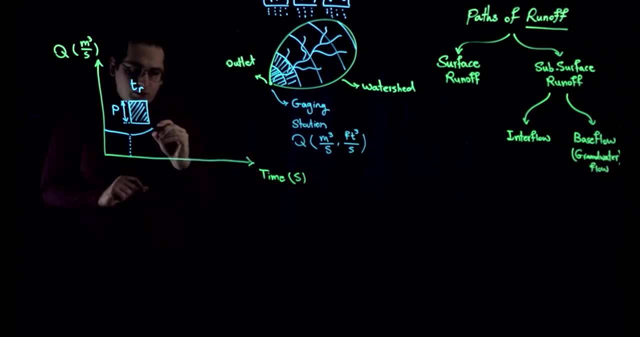 flow to the outlet. so this goes high to this point. perfect right now, because the rainfall is going to be T sub R and the height of the flow ends over here. then after that, when the entire watershed is contributing to the outlet, then the rainfall is done and it goes down like this. this point we 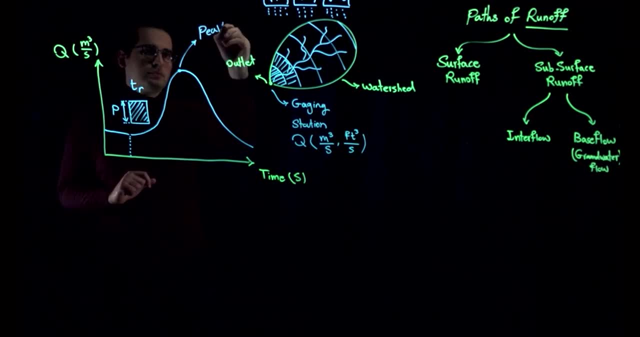 call it the peak of the hydrograph and this graph that I have shown over here, this is called the hydrograph. so a hydrograph tells you the flow of the watershed and the height of the watershed, the flow Q, at any given time- T. so there are a couple of things that I want you. 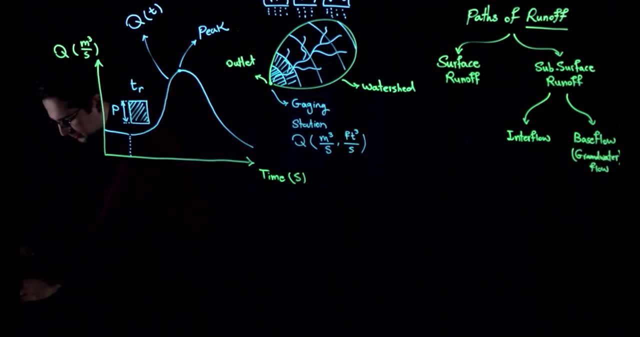 to understand when it comes to a hydrograph number one. let's see if they can, if we can, divide this hydrograph into the components that we have over here, all right. so this is the point. this is the point where a hydrograph started rising, right? if I connect this point using a straight line to the other side? 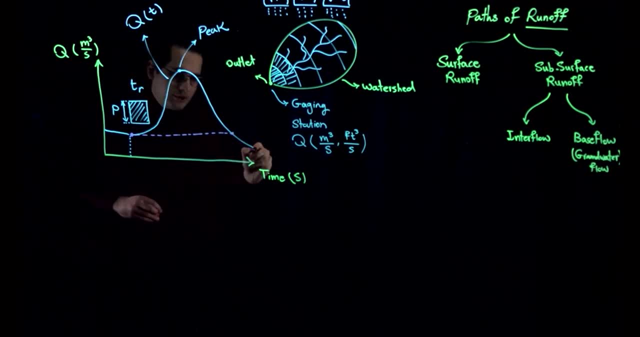 of the hydrograph, whatever is under this, which would be this area. right, this volume of water which is under my imaginary line is called base row. in other words, this base flow is the contribution of the groundwater to the stream now above the line, which would be this area. 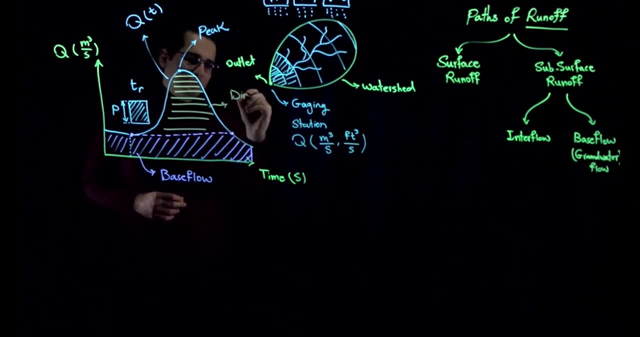 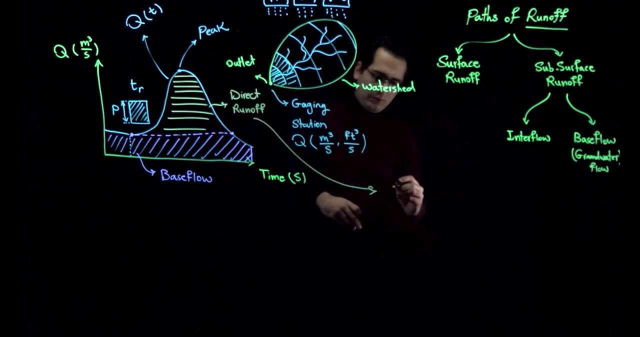 it's called direct runoff. what is direct runoff? I'm not gonna write it over here. so direct runoff is the차 nation of surface runoff and interfull. all right now. the last thing that I want to show you on this schematic figure, a schematic graph of the hydrograph, is how we can define different sections of the hydrograph. all right, so from here you can imagine this hydrograph. of the hydrograph which I'm going to read right, this pentagon is going to be. it's gonna show you two different sections of one hydrograph here at the sp backup graph line, just to estimate water, as you may have noticed on this. so the size of theлав have more than two hundred centimeters in this space, given the volumes in life you can see in nature. all right, now. now we can design open channels across per day projects which I define different infrastructure. many are in case systems, if you can't just finevel Alabama under water or a stream. so it's just a Ray Yuan. 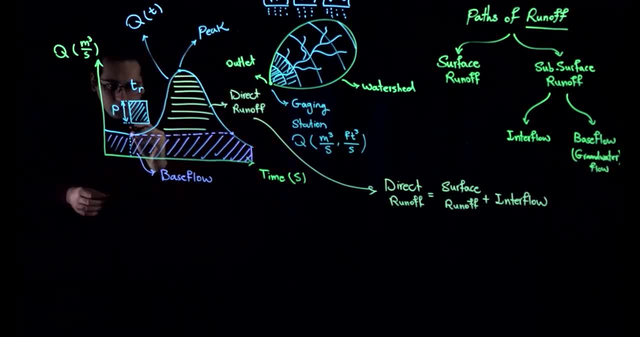 sections of the hydrograph. all right, so from here, from where the hydrograph starts to rise, all the way to somewhere over here. this part represents the rising section, or we call it rising limb, of the hydrograph. all right, so from this point all the way to a point over here.